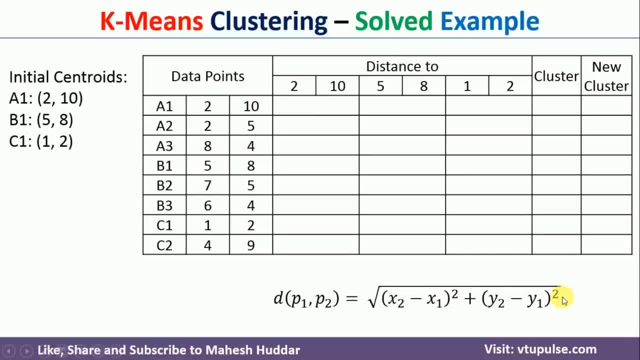 square root of x2 minus x1 bracket square, plus y2 minus square root of x2 minus x1 bracket square over here. now i will discuss how to calculate the distance between these data points to this centroid here according to this particular formula. let us assume that this particular column is x1. 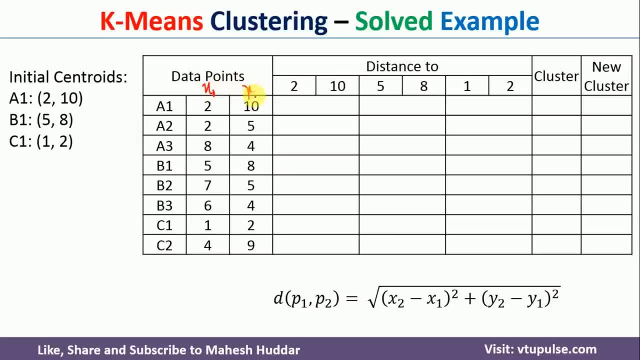 here, and this one is y1, this is x2 and this is y2. now what we can do over here is we need to put this particular values in this particular equation so that we will get the distances here. for this point a1 over here, the x? 1 is 2 and y 1 is 10. x2, y2 will remain same for this particular column here. 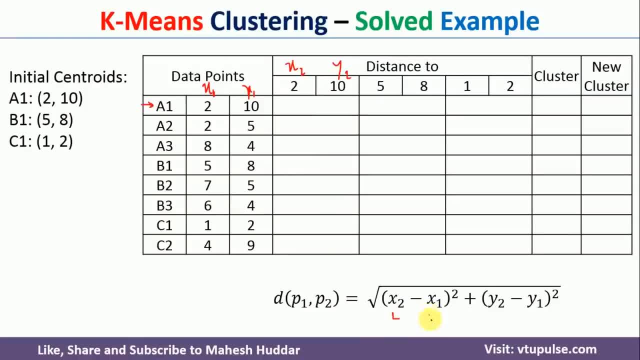 now x2 in this particular case is 2 and x1 is 2, 2 minus 2. bracket square plus. this will be bracket square over here. and then this one that is y2 is 10 and y1 is also 10 over here, if you. 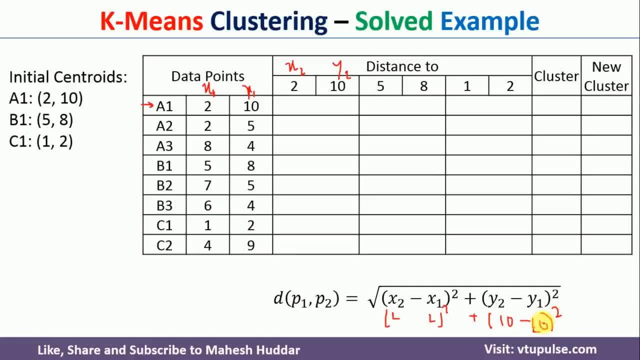 calculate this particular thing. it will become 2 minus 2 bracket square plus 10 minus 10 bracket square, that is 0. so the answer will become 0 here. so this is the finished result for this problem: will become 0. similarly, i will show one more example here. this is the another example now. 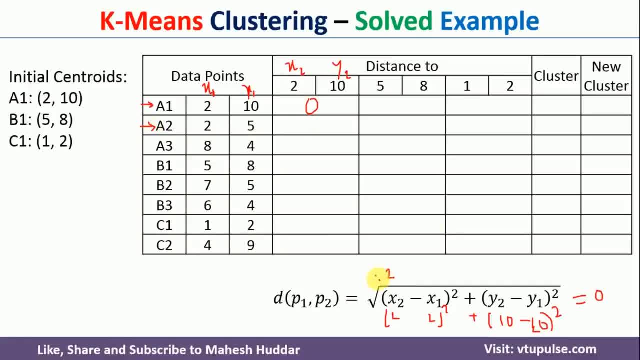 again, x2 is equivalent to what? again x2 is equivalent to 2. we have to take the square root of over here. 2 minus x1, again it is 2 bracket square plus y2. y2 is 10 in this particular case. so 10 minus 5, that is y1 is 5 over here, so that is 5. so 10 minus 5 bracket square. 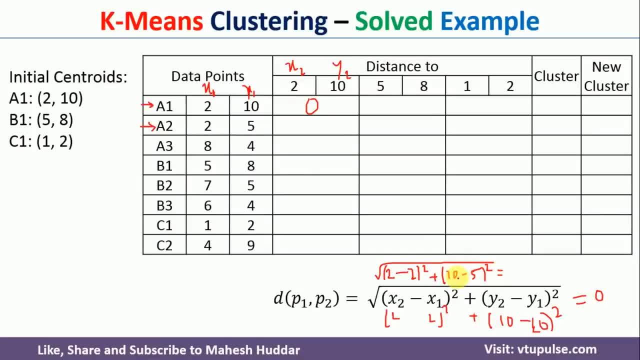 come 2 minus 2 bracket square, that is 0. 10 minus 5 bracket square is equivalent to: i think it is 10 minus 10 is. 10 minus 5 is 5. 5 square is 25. square root of 25 is again, is equivalent to 5. 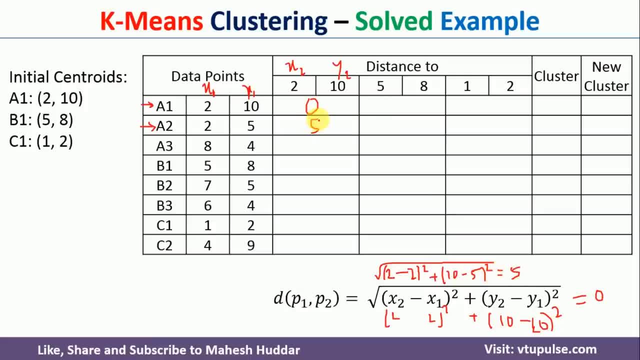 over here, so this particular data point will become 5 in this case. so, similarly, we need to calculate the distances over here. so once you calculate the distances, you will get all these values. similarly, we need to calculate the distance from this particular data point to this centroid also, as well as to this particular centroid. 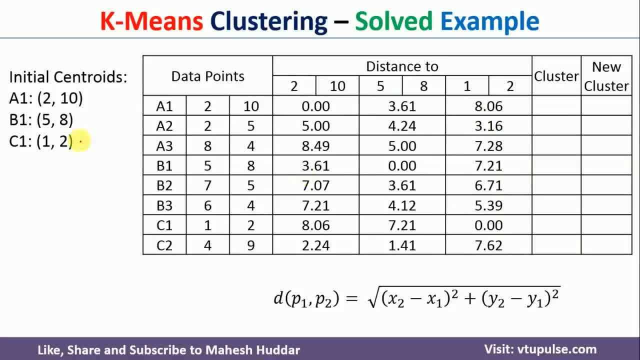 so we need to calculate the distance from this particular data point to this centroid. so once you calculate, you will get these particular values once the distance calculation is over. next, what we need to do is we need to assign these particular data points to one of these particular clusters. so what we need to do is we need to see the distances and the one which is 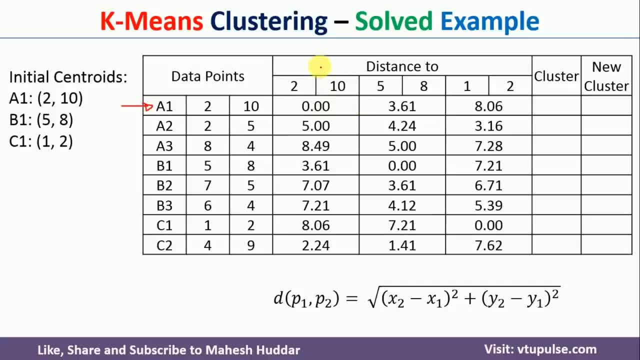 having the smallest value, to that we can assign the cluster. let us say that this is the cluster number one, this is cluster number two and this is cluster number three. if you look at these particular distances, this is the smallest one, so this particular thing will be assigned to. 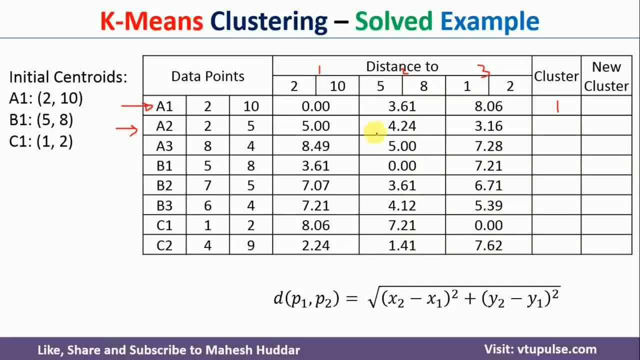 first cluster. if you look at this particular data point, you will get the smallest value and the distances are is 5, 4.24 and 3.16. so definitely 3.16 is smallest, so we will assign it to the third cluster and the same thing will be done for all the data points over here. 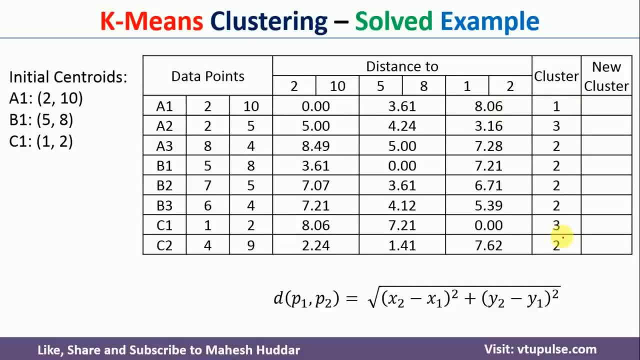 so after first iteration we will get this particular assignment over here. so first data point, that is, a1, is assigned to one. if you look at this one: a3, b1, b2, b3 and then c2 is assigned to second cluster and a2 and c1 is assigned to third cluster. over here now, once these assignments, 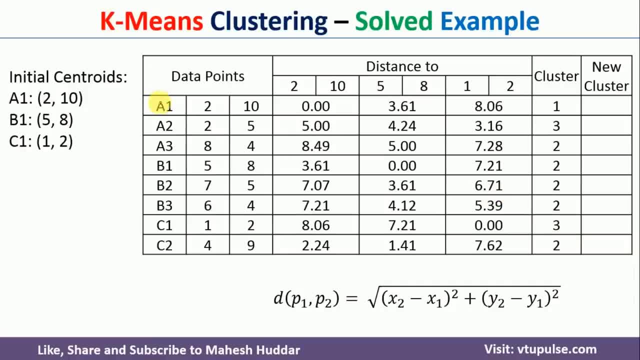 are done. now we need to calculate the new centroids here for this particular first cluster we have only one data point, so the centroid will remain same. but when it comes to second one, that is, the second cluster has one, two, three, four and five data points. so we need to take the, we need to. 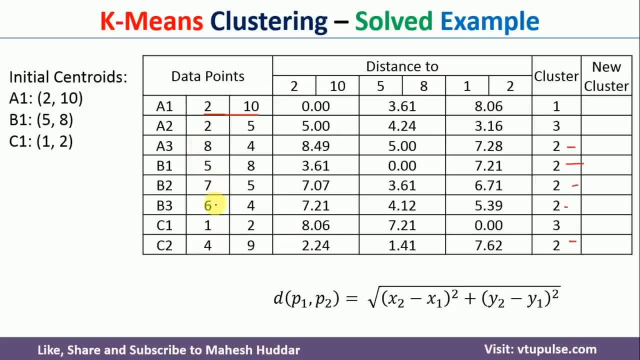 calculate the centroid here, that is 8 plus 5 plus 7 plus 6 plus 4 divided by 5.. similarly this one, that is four plus eight plus five plus four plus nine divided by five. and once you do this part, i think, for second cluster, we need to do it for the third. 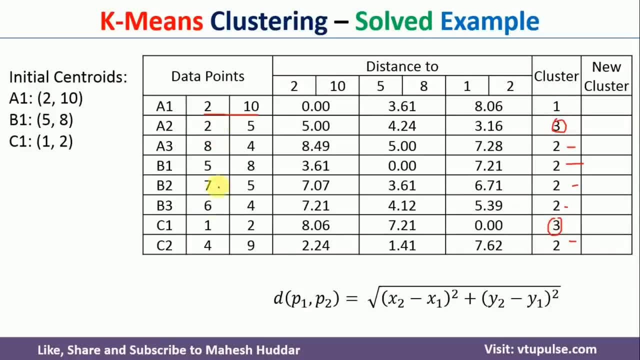 cluster also third cluster has only two data points. that is, two plus one divided by two, five plus two divided by two. that is the last one. so once you do the calculation, you will get. these are the new centroids over here. once you get this particular new centroids, we need to consider these. 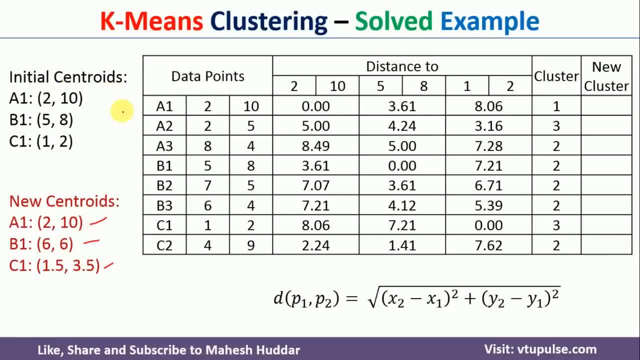 centroids as the current centroids and then we need to continue from here onwards, so i will make these as the current centroids. now we need to calculate the distance from these data points to this particular centroids. here again, i will write this particular centroids over here and then we need to calculate the distances here. so same formula we need to use. 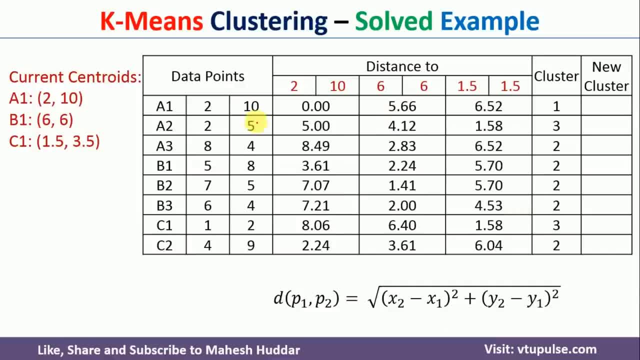 and then we need to calculate the distance. so once you calculate the distance, again we have to check which one is the smallest one out of these particular three distances. so this one is the smallest one, so it will be assigned to first cluster here between these three. this is the. 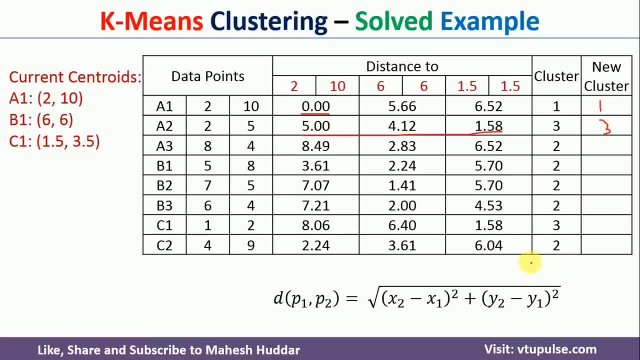 smallest one. so it will be assigned to third cluster and same will be repeated for all the data points here. now this is how the assignment takes place. this is called as a new cluster over here. now, if you look at this particular thing, in the previous case this c2 was assigned to second cluster, but now it is assigned to first cluster. the meaning: 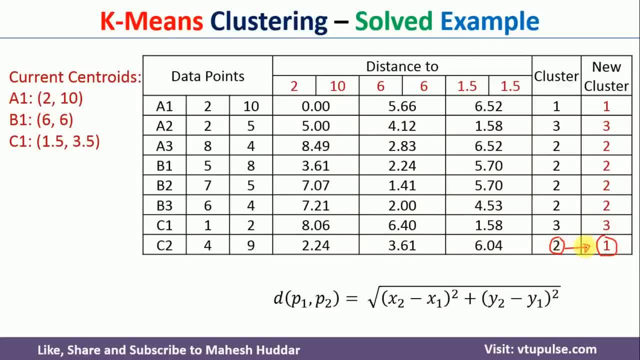 is a data point has moved from one cluster to another cluster here, so this is not at we can say that converged here. we need to calculate the new centroids again here. so how to calculate the new centroid again in first cluster we have two data points, that is, a1 and c2 here. so we need to 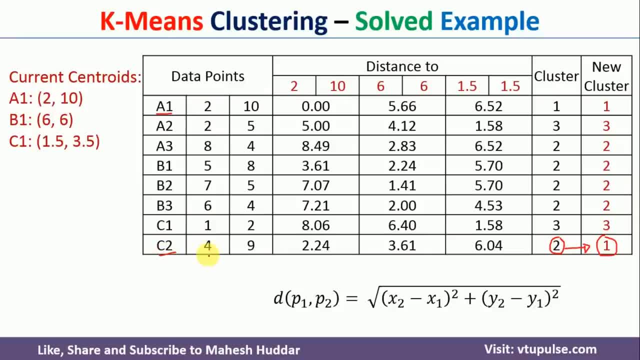 calculate the centroid of these two things. that is, 2 plus 4 divided by 2, 10 plus 9 divided by 2. that will be the new centroid here. similarly we have to do it for second cluster and third cluster over here. so we will get these three new centroids here. so once you get this particular 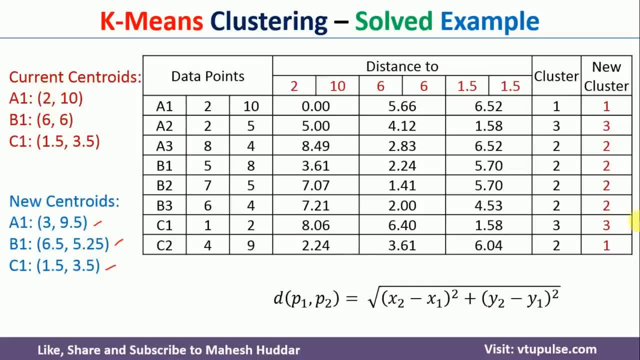 new centroid, we will consider these as a current centroids. before that, this new clusters will be come and sit over here. so that is what i have done and then we will consider this as a current centroids. from this particular data point to this particular current centroids, we will calculate. 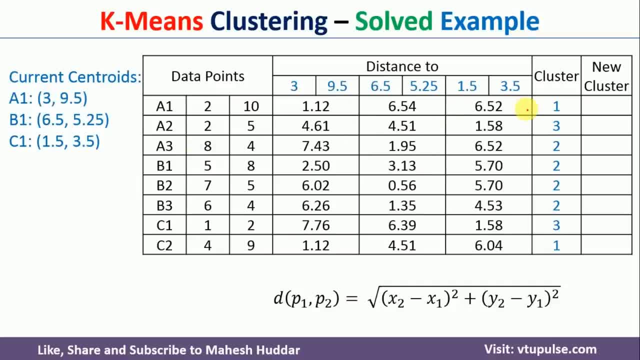 the distance is here. so once you calculate the distance again, we have to start assignment, like between these three: which is the smallest one? that is definitely 1.12, is the smallest one between these three. this one is smallest one. so this will be assigned to first cluster, third cluster and so on. so this is 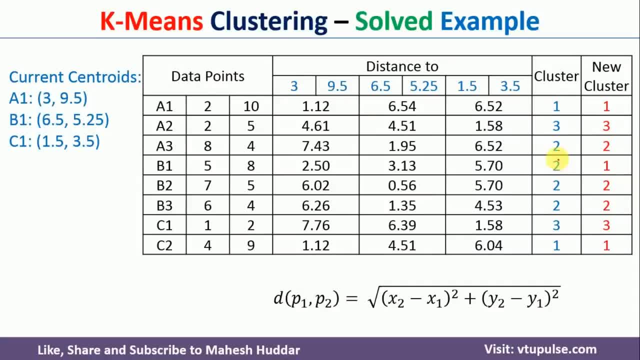 how the assignment will look like now. again, if you look at here, previously this particular data point, that is b1, was assigned to cluster number two, but now it is assigned to cluster number three, cluster number one. here the meaning of this one is again a data point has moved from one cluster to. 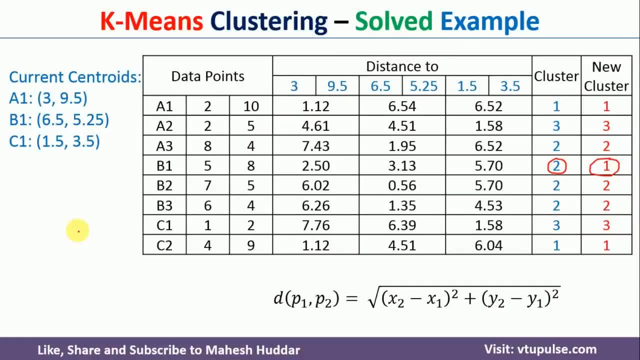 other cluster so we can calculate the distance. again we have to start assignment like between: this is a point that is control DC of this particular data on this particular cluster. so we need to calculate. the new centroid is here. so once you 될 code the new centroid, you will get something like: 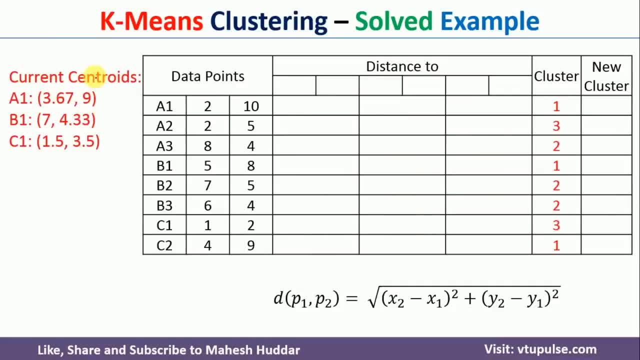 this and then this new cluster will become the current cluster here, and then we need to mixture this particular new central as the current centroid and then we need to calculate the distance to this particular centroid here. so again, once you calculate this particular distances, we have to assign this particular data points to one of this particular clusters over here. 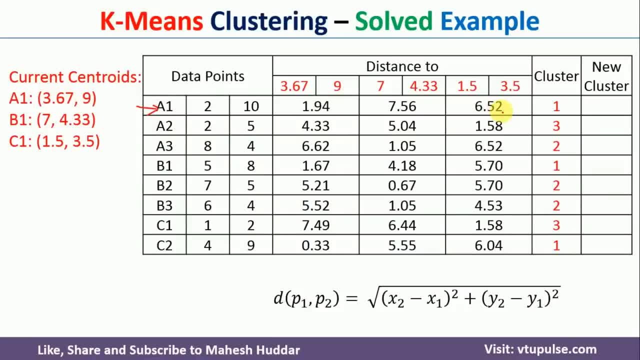 4, 7.56 and 6.52 as the distances. so this is the smallest one, so it will be assigned to one here. the same process has to be followed for all the data points. after the cluster assignment. it looks something like this, and if you compare the previous assignment and the current assignment, both are: 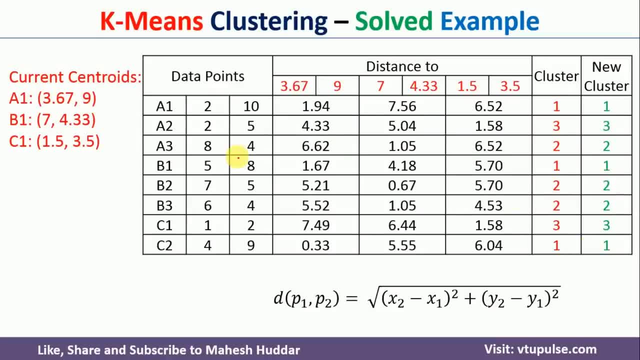 exactly same here. it shows that all the data points have converged to these particular new clusters here. so once that is done we need to write down the final clusters over here. the final clusters are this particular a1 belongs to first cluster, b1 belongs to first cluster and c2 belongs 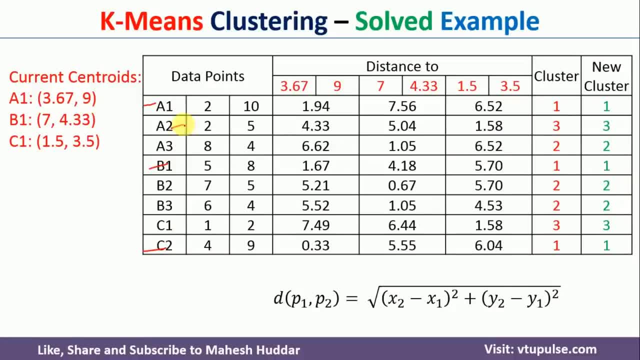 to first cluster over here. similarly, this a2 and c1 belongs to third cluster remaining, that is, a3, b2 and b3 belongs to second cluster over here. so this is how, actually, we can easily use the k-means clustering algorithm with the euclidean distance to divide the data points into different. 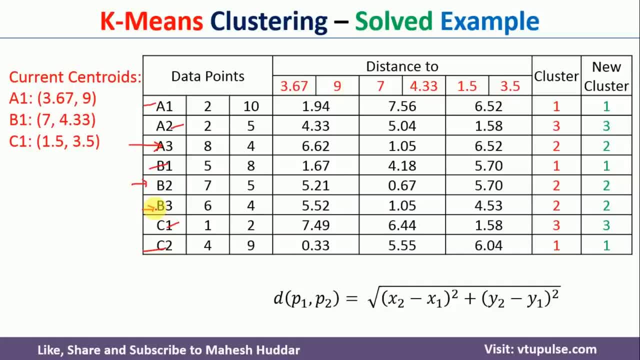 clusters here. i hope the concept is clear. if you like the video, do like and subscribe to my channel and hit the bell icon so that you don't miss any of my new videos. so share with your friends. press the subscribe button. for more videos, press the bell icon. for regular updates. thank you for watching. 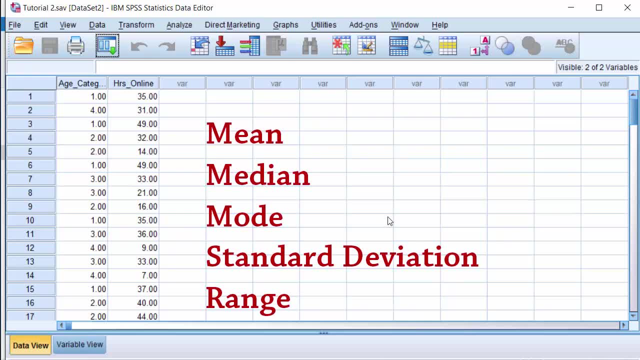 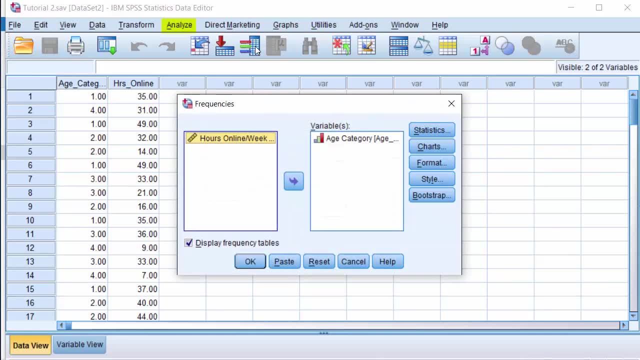 To obtain Mean, Median Mode, Standard Deviation and Range in SPSS: click Analyze Descriptive Statistics- Frequencies. I'm going to click Reset here to set selections to their defaults. Let's put ours online. in the variable list, Click Statistics. 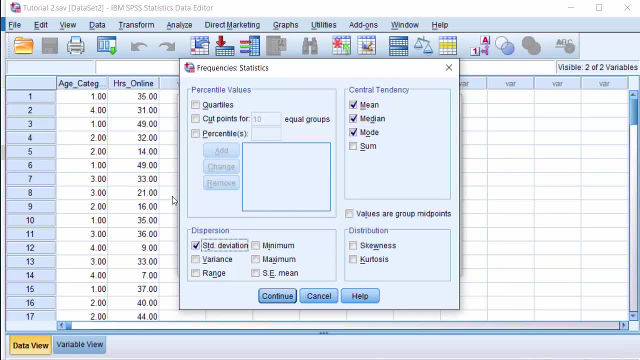 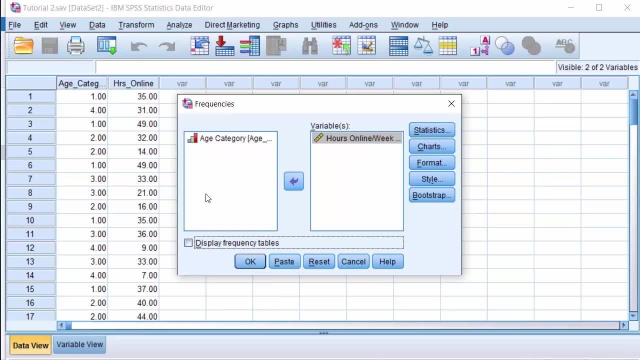 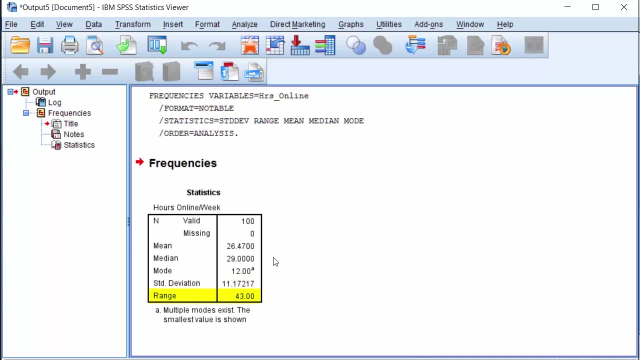 We want Mean Median Mode Standard Deviation and Range. Click Continue. Uncheck Display Frequency Tables, since we don't need them now, And click OK. And here we have the Mean Median Mode Standard Deviation and Range.